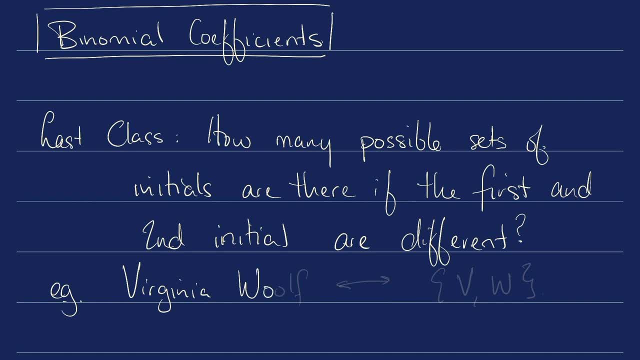 So, if you have a name like Virginia Woolf, what we're talking about is creating a two-element set made from letters, where the first and second elements have to be different from each other. In order to answer this question, the first thing that we need to do is clarify. 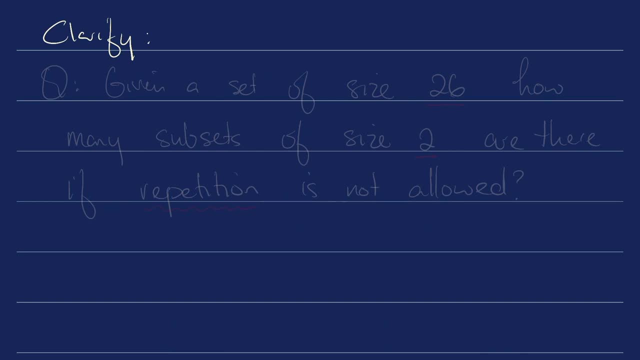 We can clarify this question and start to answer it by realizing what we're actually talking about. So the question is asking: given a set of size 26, the letters, how many subsets of size 2 are there? if repetition is not allowed, This is: the same question we were asking in the first class. So if you have a set of letters, how many subsets of size 2 are there if repetition is not allowed? This is the same question we were asking in the first class. So if you have a set of letters, how many subsets of size 2 are there if repetition is not allowed? This is the same question we were asking in the first class. 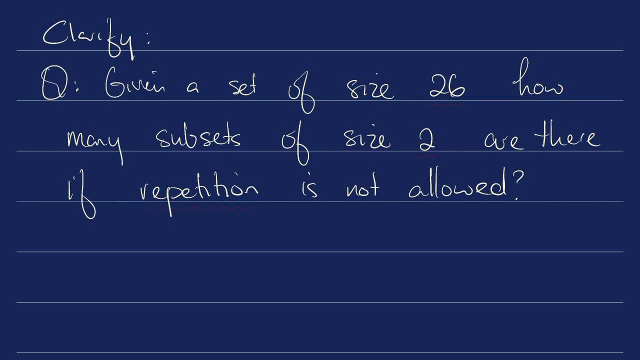 So if you have a set of letters, how many subsets of size 2 are there, if repetition is not allowed? This is the same question we were asking in the first class, But using the language of sets and subsets. After we clarified, the next thing that we can possibly do is generalize. 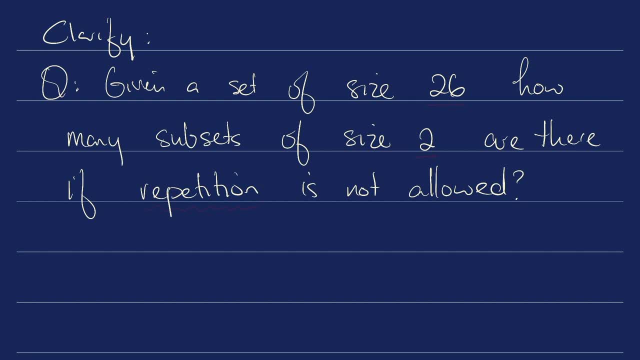 Mathematically speaking, it's always good to generalize what you're talking about. So here I have a set of 26. It didn't really need to be 26.. And here I have a set of size 2. It didn't really need to be 2.. And there's this concept of repetition. 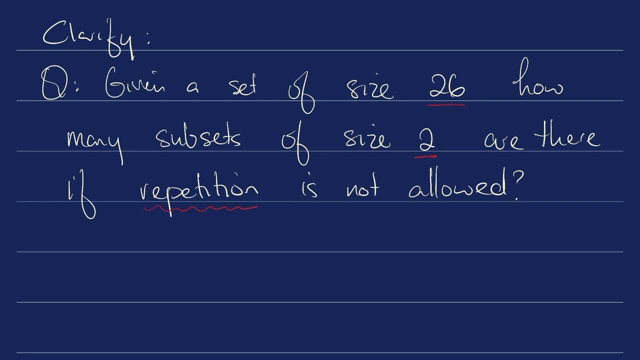 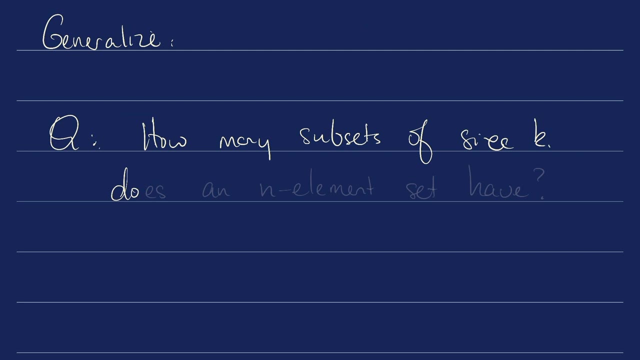 And we can realize that the concept of sets already takes into account the fact that repetition is not allowed. So we can generalize the question to say how many subsets of size k does an n-element set have? Starting with our original question about initials, we can clarify and generalize it to: 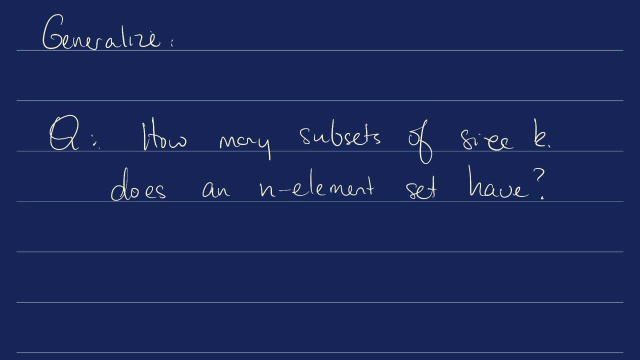 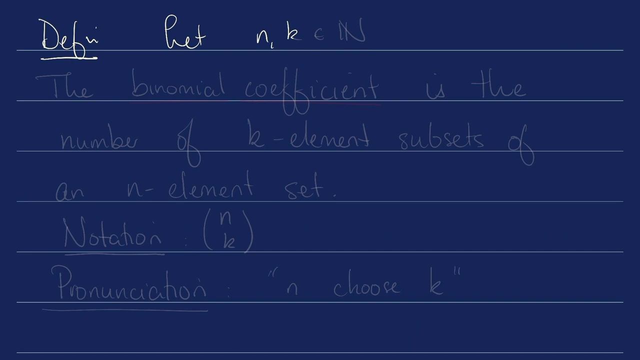 this question. Really, underneath it all, we're asking: how many subsets of size k does an n-element set have? In order to answer this question, we introduce the notion of the binomial coefficient definition. So first, let n and k be natural numbers. The binomial coefficient. 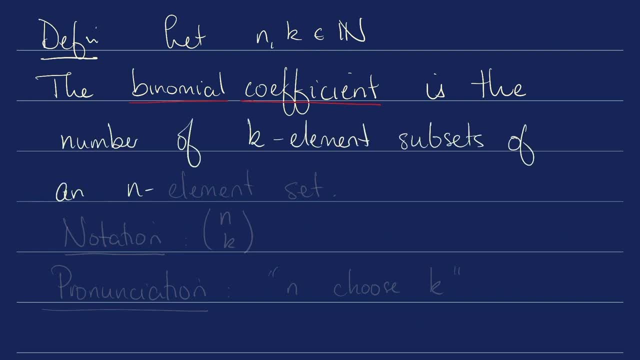 is the number of k-element subsets of an n-element set. The notation for this is the two numbers that act on top of each other, between parentheses- n above and k below, And the way you pronounce it is n. choose k Then out of a set of size n. how many ways can you choose k things? 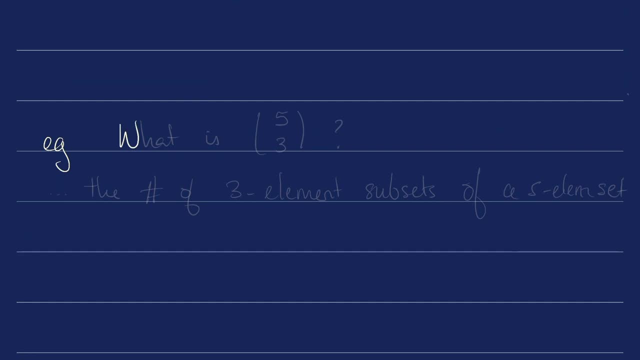 Let's do an example Example. What is 5 choose 3?? Remember, this is asking the number of 3-element subsets of a 5-element set. Let's just write some things down. We're going to need a little bit more space. 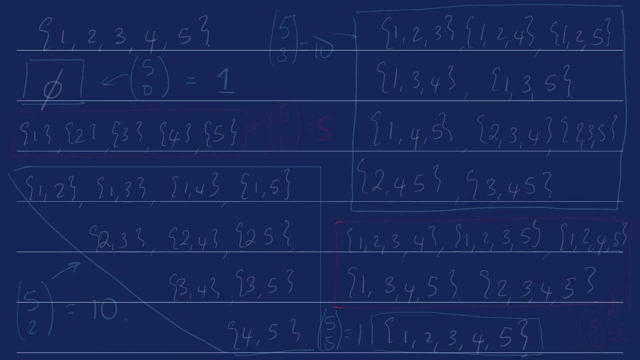 So we're going to start with our 5-element set and we're going to label all of the possible subsets. So we're going to label all the possible subsets and I'm going to organize by size. So here we go. There's the subset of k. 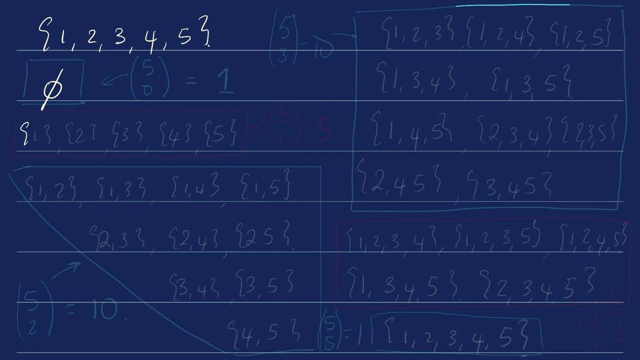 There's the subset of k-0.. Then we have the subsets of k-1.. The subsets of k-2.. The subsets of k-3.. the subsets of cardinality four and the subsets of cardinality five. All right, let's talk about this. This is going to be. 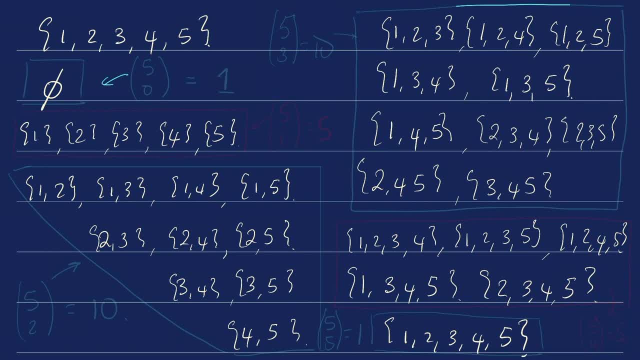 five choose zero Out of a set of five. how many ways can you choose zero things? Only one way To get the empty set. So five choose zero is going to be one. Here are all the ways to choose one thing out of a set of five. So this is five choose one. 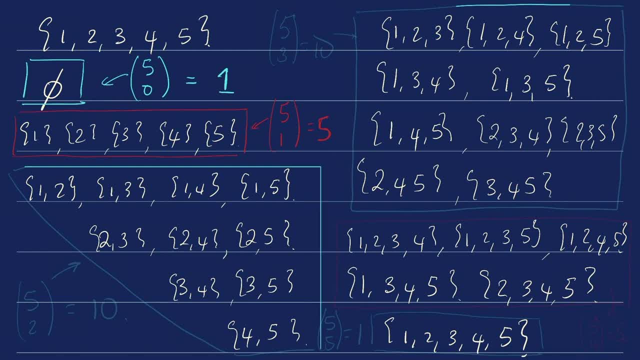 and it is five. This is all the ways to choose two things out of a set of five. So this is five, choose two, and it is ten. Here are all the ways to choose three things out of this set of five. So this is five, choose three, and it is also ten. Here are all the ways to choose four things. 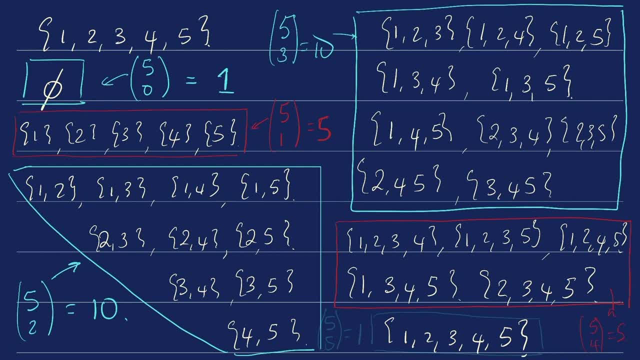 and this is five. choose four, which is five. And, last but not least, this is the only way to choose five things. So this is five, choose five, which is one. As of this point, these numbers might seem a little random. 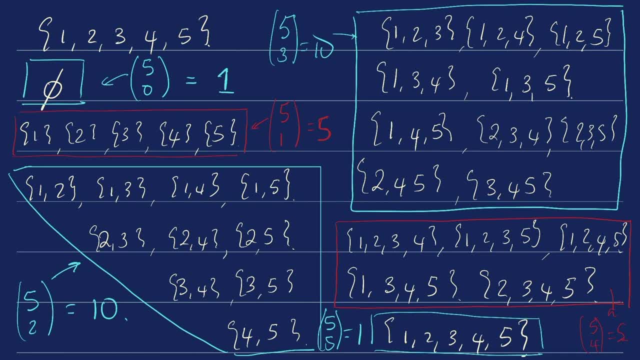 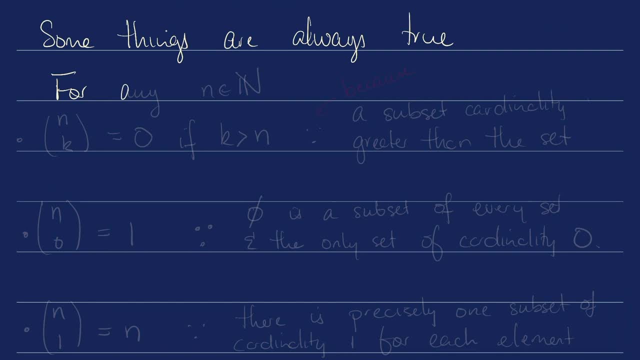 But that's not actually the case. Some things are always true about binomial coefficients, and some of these things are also not too complicated to explain. So for any natural number, n, what is going to be n? choose k. when k is greater than n, Well, it's going to be zero. 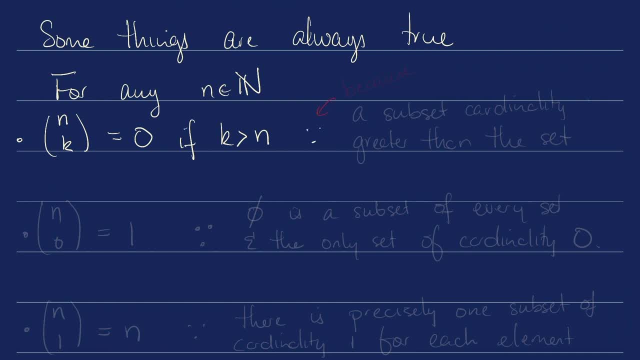 because- and this is the notation for because- because a subset, a subset, cannot have cardinality greater than the set that you started with. So if k is greater than n, how many ways can you choose k things out of a smaller number of n things? It's zero. There is no way to do that. What about? 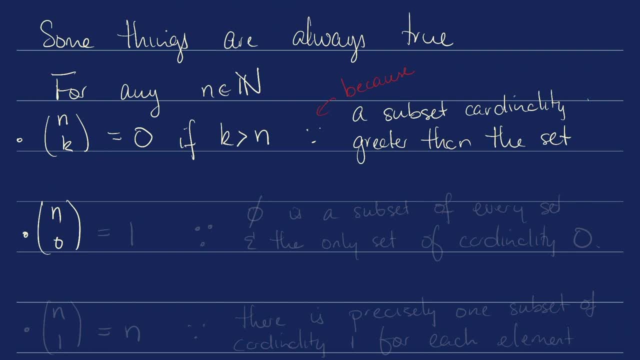 n choose zero. How many ways can you choose zero things? Only one way, no matter what n is, because the empty set is a subset of every set and the only set of cardinality: zero. Last but not least, n choose one. no matter what n is, is going to be n. 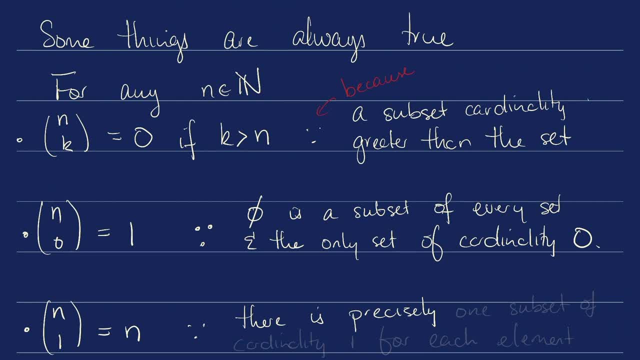 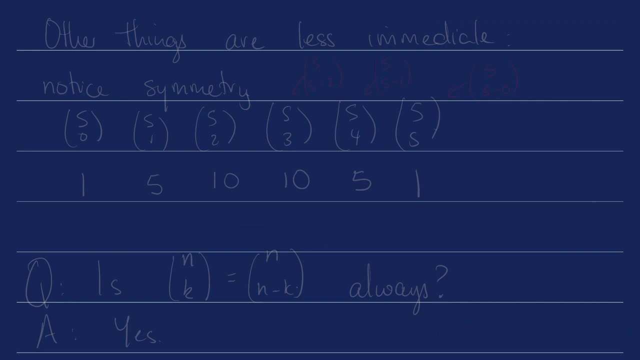 because there is precisely one subset of size, one of cardinality, one for each element of the set. How many ways are there to choose one thing from a set that contains n elements? Well, there are n ways to do that. There are some other things that are true but are more difficult to explain, But we're going to try. 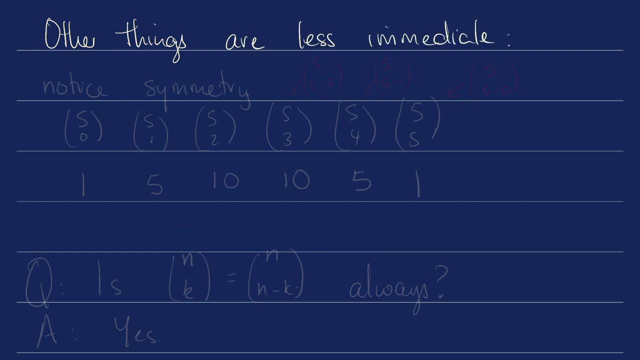 So other things are less immediate, But let's try and explain them. So notice the symmetry. So 5 choose zero, then 5 choose one, 5 choose two, 5 choose three and 5 choose four and 5 choose five. 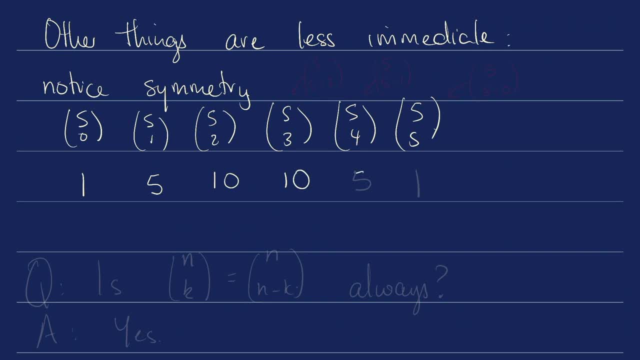 This is going to be one: 5,. ten, ten, five and one. Here's something that might make this easier for you to think about, easier to parse. Notice that this is 5- choose 5 minus 0, and this is 5- choose 5 minus 1,. 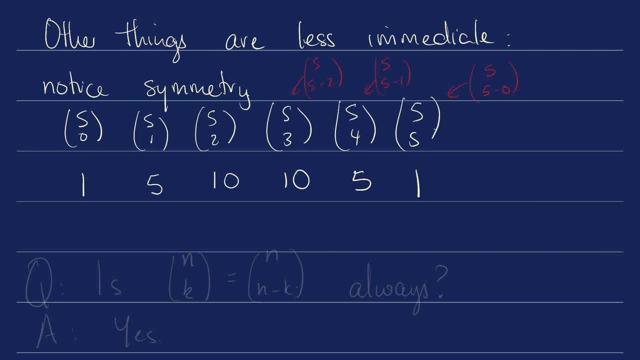 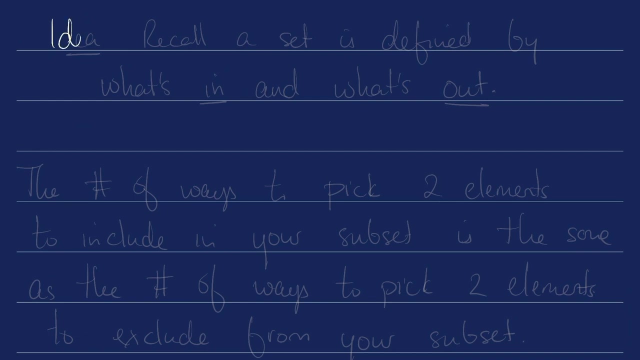 and here is 5 choose 5 minus 2.. So what we've shown is, at least in this example, that n choose k is equal to n choose n minus k, and the question that we have is: is this always true? The answer is yes. Let's explain why. 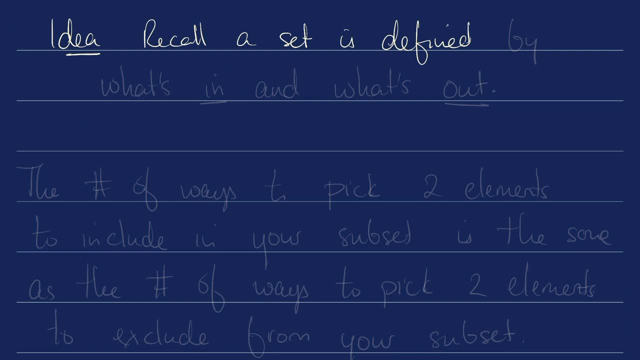 Here's the idea. Remember that a set is defined by what's in and what's out, and the number of ways to pick two elements to include in your subset is the same as the number of ways to pick two elements to exclude from your subset. 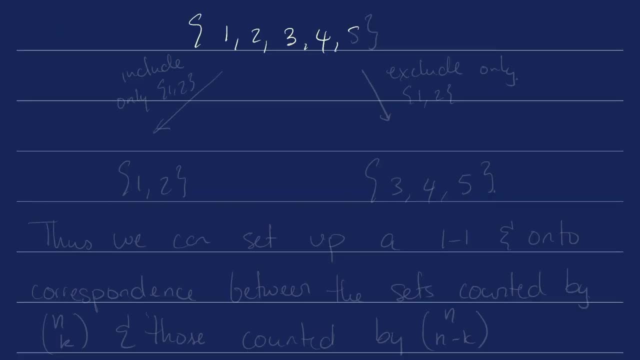 Let's talk about, say, a set of 1,, 2,, 3, 4, 5.. You can choose to include 1 and 2, or you could choose to exclude 1 and 2.. If you choose to include 1 and 2, you'd get the set one. 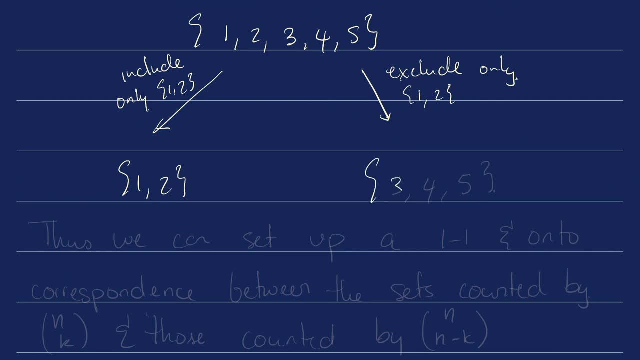 complex set a 2. If you choose to exclude 1 and 2, you'd get the set 3,, 4,, 5. And we are setting up a correspondence between these two sets so that we know that for every one of one kind there's going. 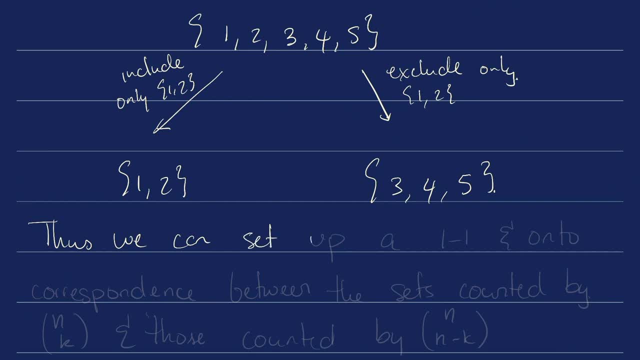 to be one of the other kind. Thus we can set up a one-to-one and onto correspondence between the sets counted by n choose k, which is, you know, include choose k things to include in your set, and the sets counted by n choose n minus k, where you choose k things to exclude from your set. 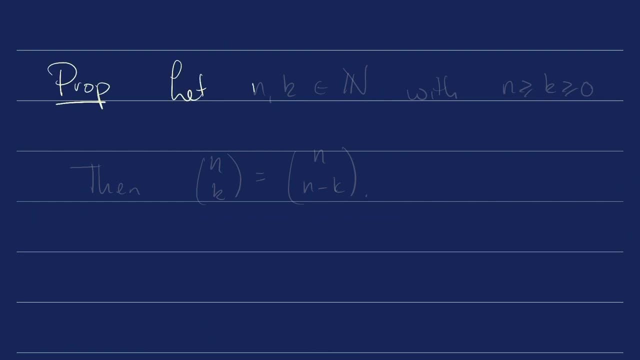 Said formally. here's our proposition: Let n and k be natural numbers, with n greater than or equal to k greater than or equal to 0. Then n- choose k is going to be equal to n. choose n minus k- Great. Let's explore some other formulas involving our binomial coefficients. So here's a. 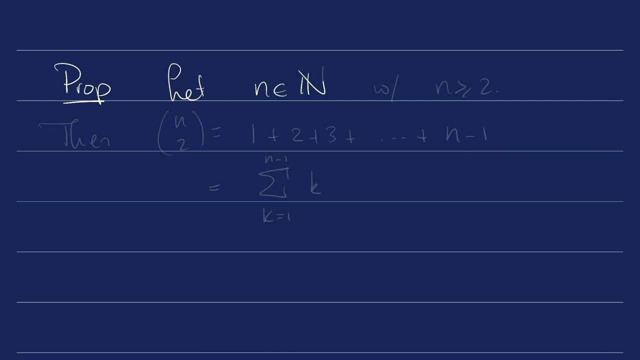 proposition. So let n be a natural number with n greater than or equal to 2.. We are going to claim that n choose 2 is equal to 1 plus 2 plus 3 plus all the way up to n minus 1,. 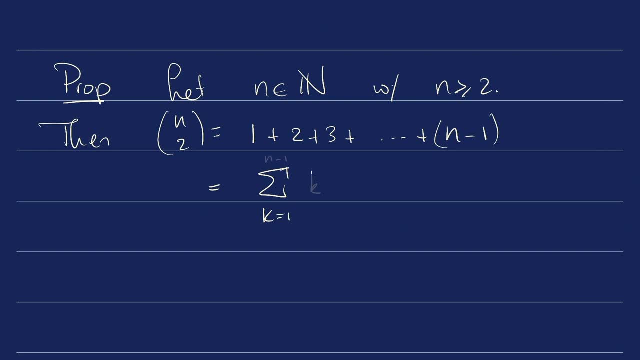 which said otherwise or written otherwise is just this sum, The sum of k, as k goes from 1 to n minus 1.. The idea behind this and the reason that I want to go through this is because there is a common way of approaching combinatorial proofs. So the sum of numbers on the right hand side of that, 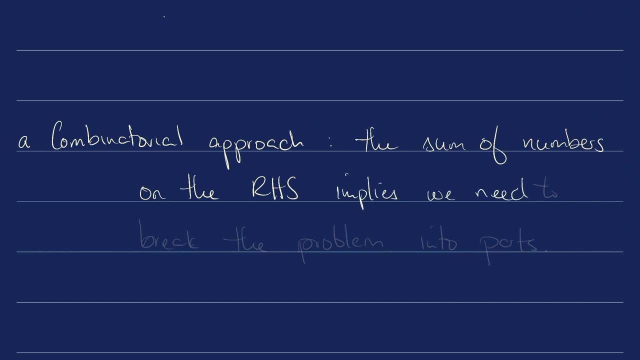 equation implies that we we need to to break the problem into parts. How do we break down whatever n choose? to k means into things counted by one and then two and then three, etc. Here's the idea I have here. So there are going to be n minus 1, two element. 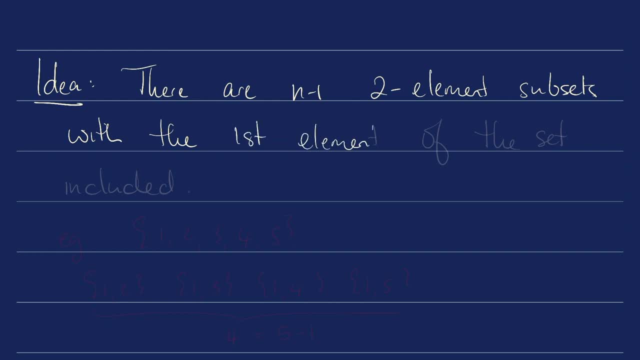 subsets with the first element of the set included. So, for example, if you start with the set 1 comma 2 comma 3, comma 4, comma 5, you know we've got 1, 2, 1 3, 1 4, and 1 comma 5.. So there are 4 is equal to 5 minus 1. 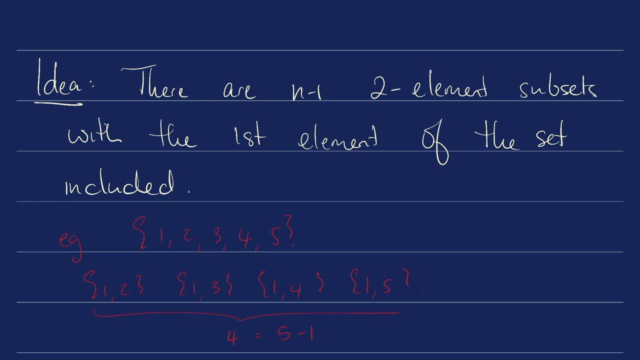 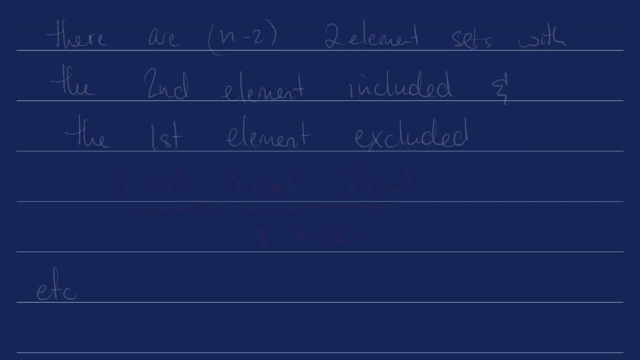 two element sets with which has number one included, and kind of: we can set up a pattern this way: So there are n minus 2, two elements sets with the second element included, But we already have all the sets that include the first element. so we're going to exclude the first element. So in our example, 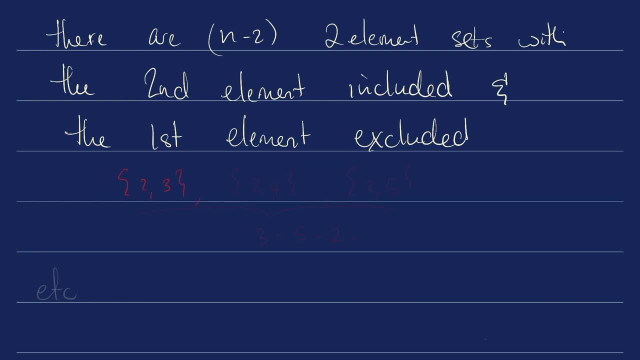 this is going to be 2 comma 3,, 2 comma 4, and the set containing 2 and 5.. And there, how many of them are there? There are three, which is 5 minus 2.. We're going to